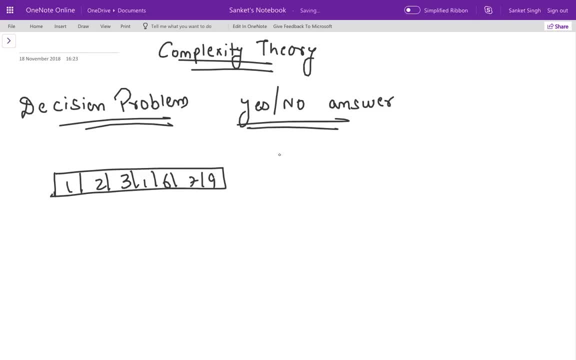 So a decision problem can be to detect if there is any integer That is present more than once. So here in this input, as you can see, 1 is present more than one time, So the answer will be yes. 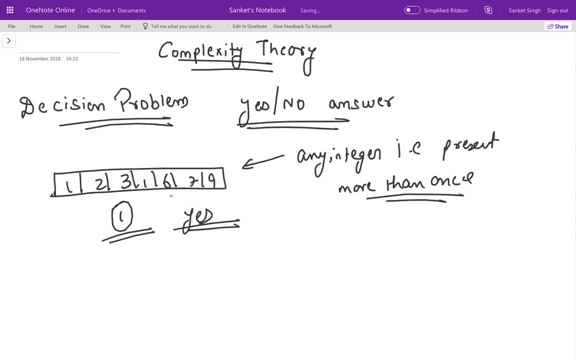 So decision problem is defined as the class of problems which has a yes or no answer associated with it, depending on the input values. So whatever the answer will be, it will depend on what the input will be given. So it will look like this that a decision problem will get some input and give a yes or no answer corresponding to it. 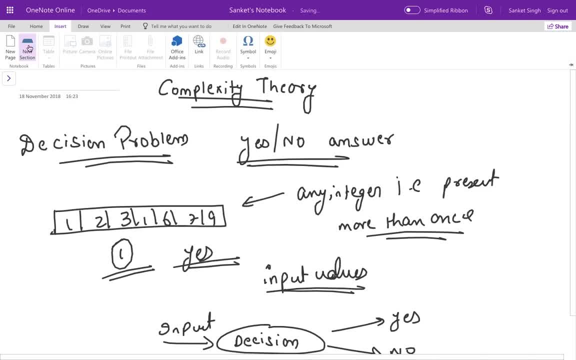 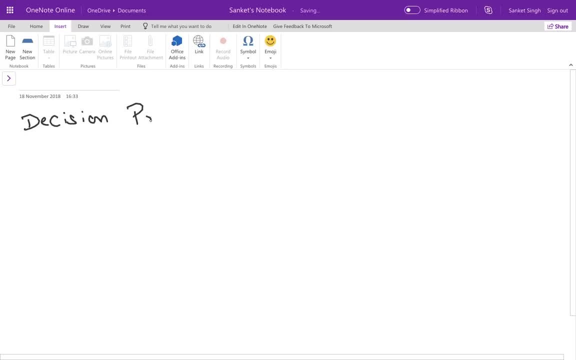 And now let us define what is decision procedure. So a decision procedure is associated with a decision, with a decision problem. So for a given decision problem, if we assume that we have an algorithm for solving it, the process of solving such a decision problem into a form of algorithm. 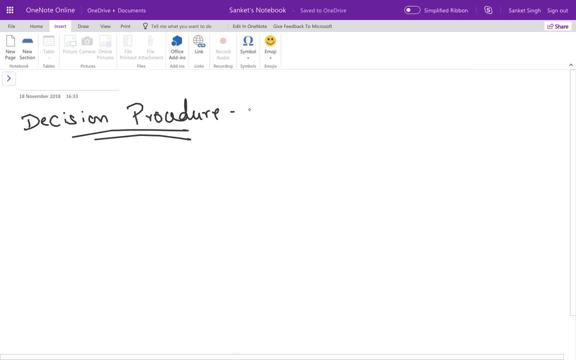 is known as decision procedure. All I want to say here is that for a decision problem, if we are solving it by any algorithm, then the process of solving this decision problem is known as decision procedure. So I hope you all have understood what a decision problem and what are. 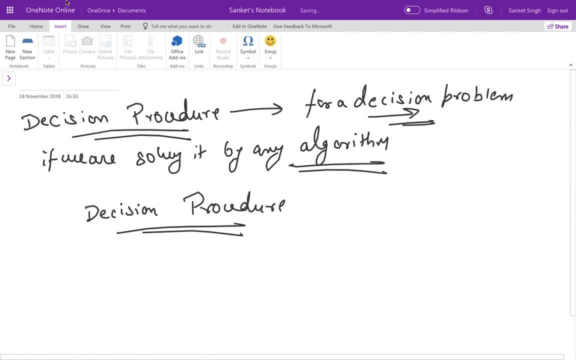 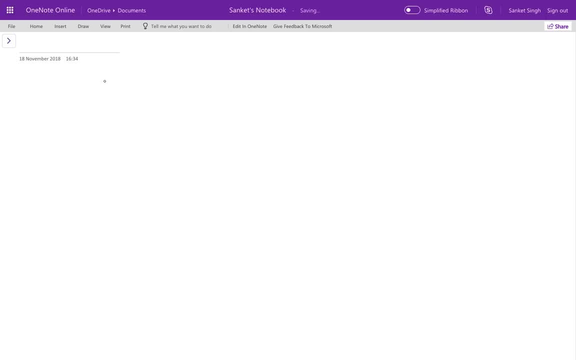 decision procedures are. So now let us define our complexity classes. So, as you all know, in our modern day computer science we deal with many kinds of problems. So if a problem has a particular algorithm, then we can say: this problem is solvable. and for an algorithm to solve a particular problem, this algorithm should give us the 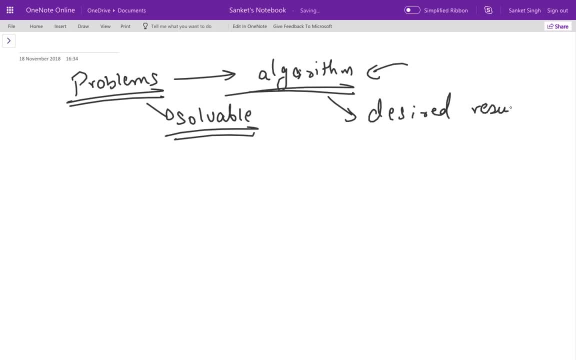 desired result in some expected amount of time. So complexity classes deals with the theory of computation that studies the resources required during the computation of a given problem. What I want to say is that if we are able to describe what resources will be required to solve, 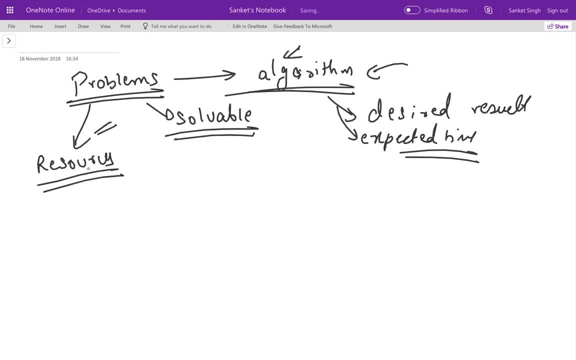 this problem using this particular algorithm, then this study will be included in the complexity theory. And currently the complexity classes can be defined into various types, Types of complexity classes. So there are many complexity classes. The first is p-class. So what is a p-class? The p-class is a set of decision problems. 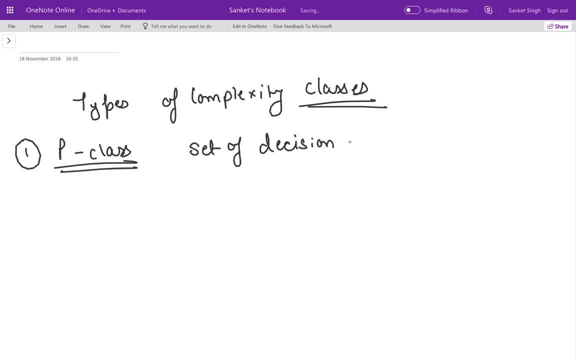 These are the types of complexity classes that are defined in the complexity theory. These are a set of decision problems that can be solved by a deterministic machine in a polynomial time. So if there exists any algorithm to solve a particular decision problem in polynomial time, then we will say that this particular problem lies in the p-class. So if there exists, 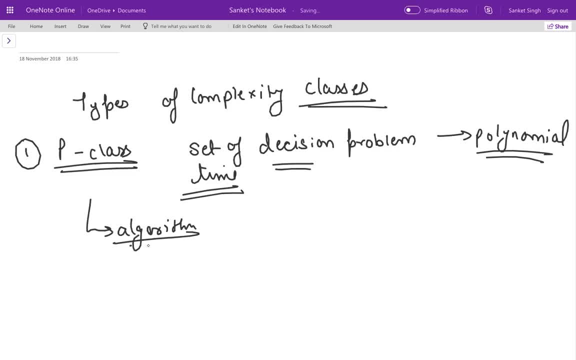 any algorithm which computes the solution to this particular decision problem in big O of n to the power k time, where k is a constant and n is a factor dependent on input, dependent on input size. So if we are able to deduce any algorithm that can solve this decision problem in big, 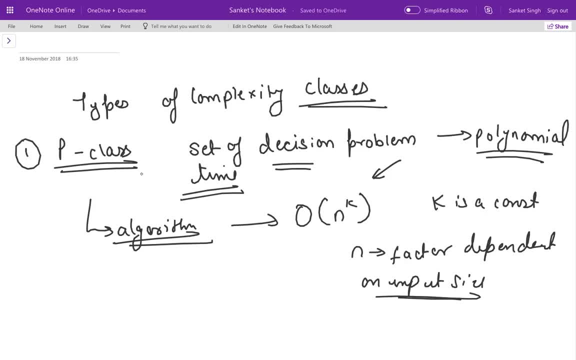 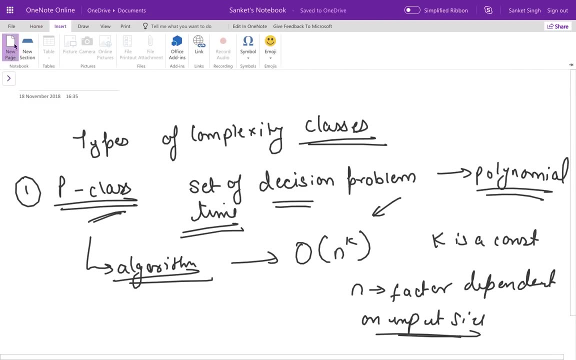 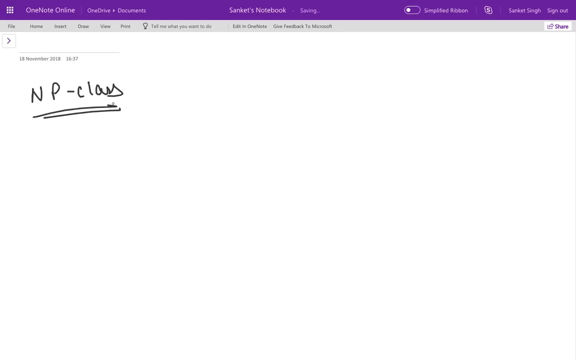 O of n to the power k time, then we will say that this particular problem lies in the p-class. So p-class has the set of decision problems that can be solved in polynomial time. So now let us define what are NP classes. So the complexity class, NP, stands for non-complexity class. 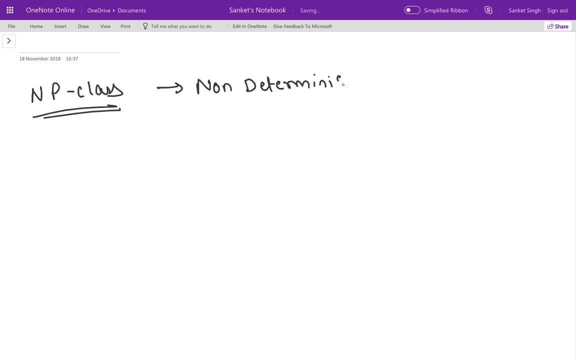 So the complexity class NP stands for non-complexity class. So from next slide we will look again at the NP class. So it stands for non-deterministic polynomial class. these are set of decision problems. these are set of decision problems that can be verified in polynomial quality. 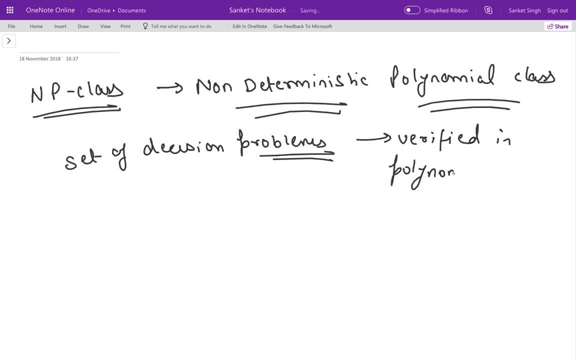 polynomial time. so what I am trying to say here is: suppose for a given problem, if it is solvable in polynomial time, then it lies in the P class, and if a problem is verifiable, then it lies in the NP class. so what I mean by saying a? 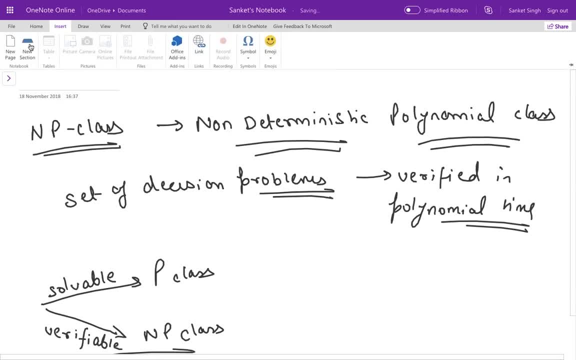 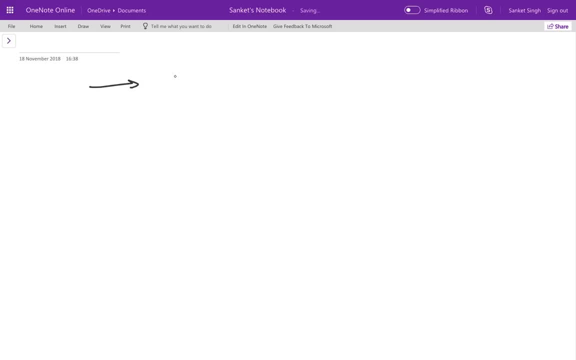 problem is verifiable. so let us take an example. suppose we are given a problem, like we have 500 students in a school and suppose we have 100 rooms available in a particular school. so a selection of 100 student must be, pay must be done for accommodating these 500 students into these 100 room. so what we have to do 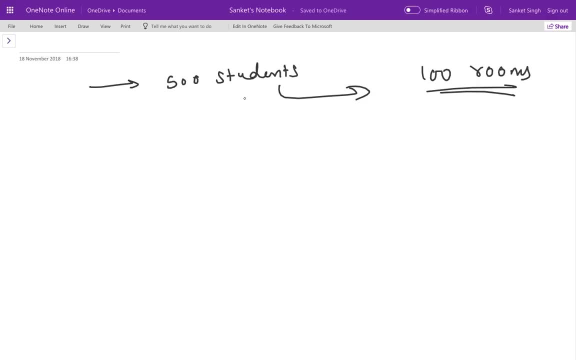 here is make some combination such that we can accommodate all these students in this particular hundred rooms, but there are certain certain conditions that few students should not be grouped together. so, as you can see, the total possible pairing will be very, very large. the total possible permutations for pairing of these 500 students, keeping info in mind, 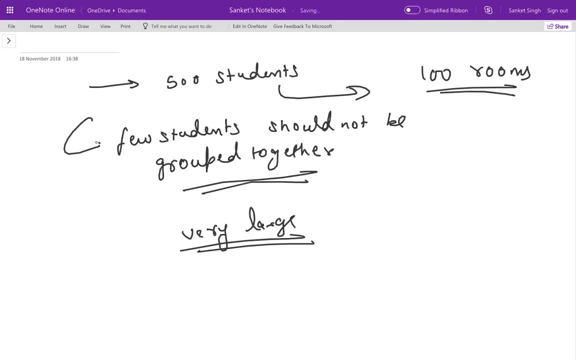 about the fact that few students should not be grouped together will be still very large. so computing these many combination will be a very heavy task. so computing these many combinations will be a very heavy task. these combinations will be a very heavy task, but if we have the solution, but if 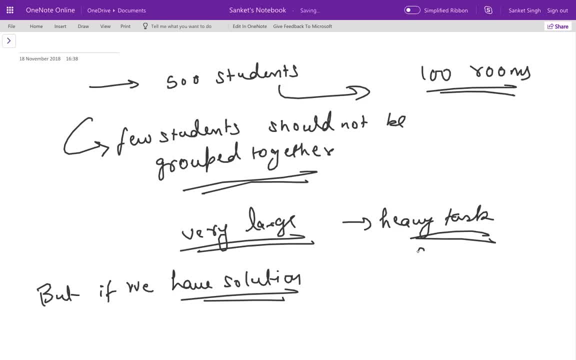 we have the solution that someone gave us all the possible combination for accommodating these 500 students into these hundred rooms, then we can easily verify that if this condition is satisfied or not. so checking that these few students are not grouped together can be done in polynomial time, so what? 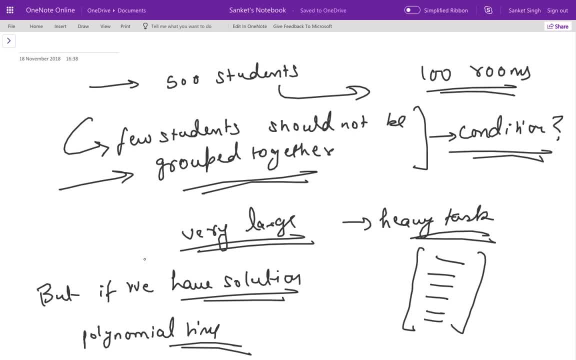 I'm trying to say is if someone gives us a solution to the problem, we can tell them that, whether it is right or not, in polynomial time, as the total possible number of pairing is too large in this particular problem, but the number of possible pairs that are prohibited to live together are quite countable. so we 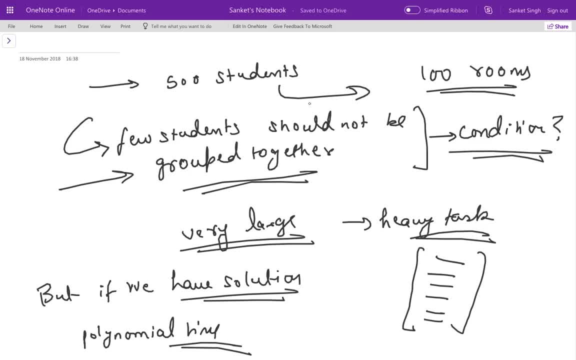 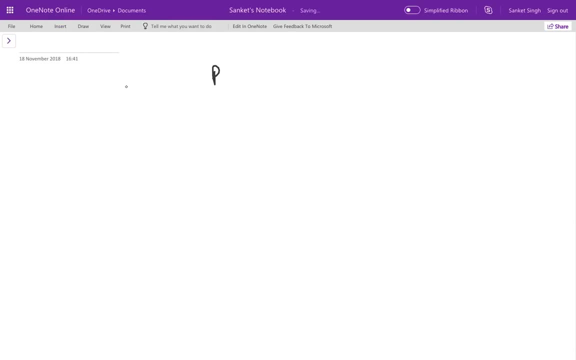 can see that every possibility of not of these students not getting grouped together in polynomial time. so let me, let me summarize this, so what I am trying to say. if, for example, if someone gives us a solution to the problem, we can say that if for a decision problem. if for a decision problem, if we are able to. 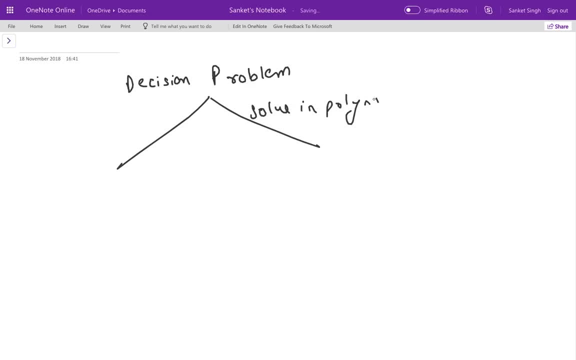 solve in polynomial time, then these lies in the P class. else, if we are able to only verify- not solve but verify- in polynomial time- then these lies in the NP class. so, as in the previous problem, the total number of combinations were very large, but the total number of restrictions that need to 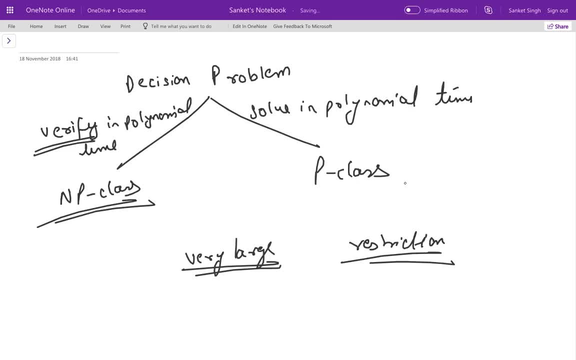 be checked were quite considerable. so we were able to verify the problem in polynomial time. so I hope you all have now got a clear perspective of what P class is and what is a polynomial time, what NP class is. and now let us define one more complexity class called as co-NP. 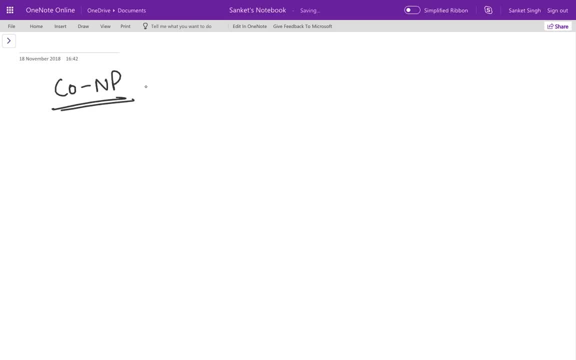 so what co-NP is? co-NP is just opposite or complement of NP, so NP class problems were able to verify only those which give answer yes. so what I am trying to say is that only yes answers are polynomial time verifiable. and if polynomial times are verifiable, then if 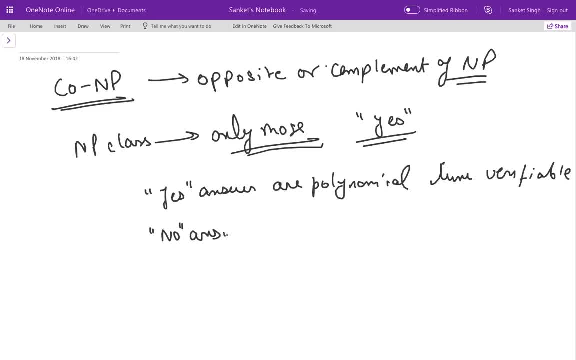 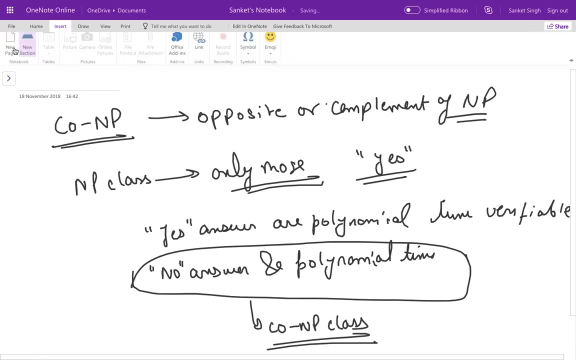 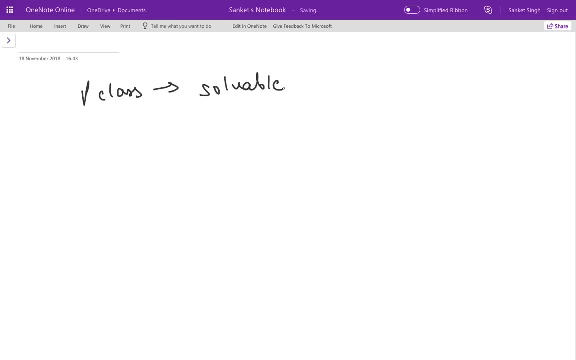 we have to verify all the no answers and we can do this in polynomial time. then these set of problems that are giving us no answer and can be verified in polynomial time lies in the co-np class. so what we have studied, still study. until now the P class is solvable. 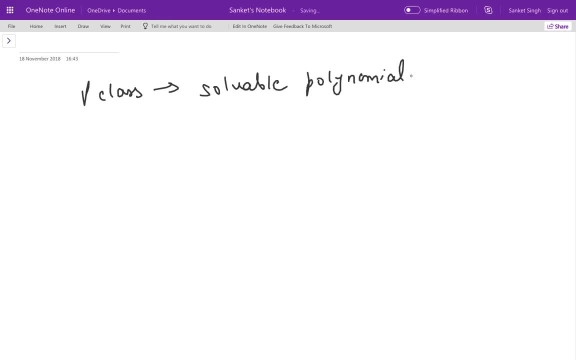 in polynomial time. the NP class is: if yes answers are there, then we can verify in polynomial time. Get to know how to solve the polynomial. okay, sir, polynomial time and for co NP class, all the no answers will be verified in polynomial time. so what will be the relationship between the above three? 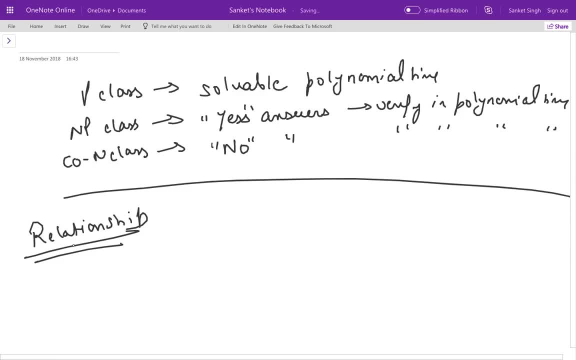 classes. as you can see, if we are able to solve any decision problem in polynomial time, then isn't it obvious that if a problem is solvable in polynomial time, then obviously we can verify. we can verify also this particular problem in polynomial time, whether the answer is yes or no, in both the condition if a problem was already. 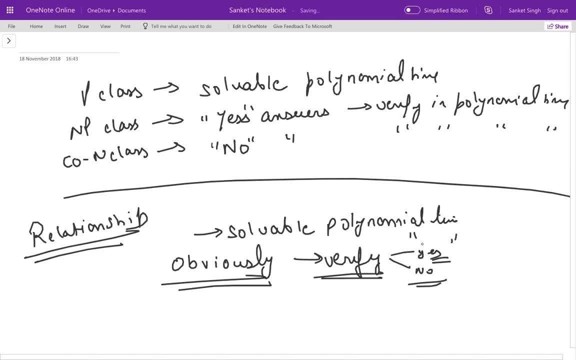 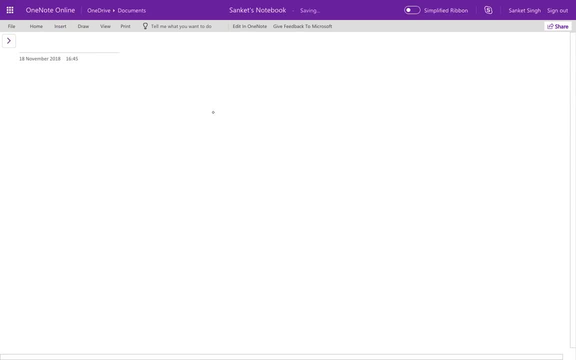 solved in polynomial time, then it can also be verified in polynomial time. so the relationship between P class, NP class and co NP class will look similar to this, where this will be a Venn diagram and this area will represent NP class, this area will represent co NP class and 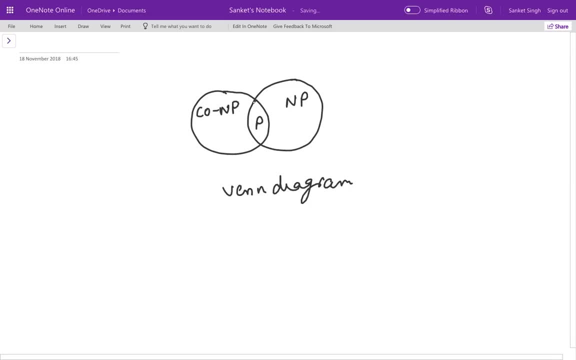 this will represent P class, as I have shown here, the P class as intersection of both NP and co NP classes, because the NP classes were those problems for which, if there is an answer yes, then it can be verified in polynomial time, and for co NP, if the answer is no, then it can be verified and for a p class problem it is already solvable. 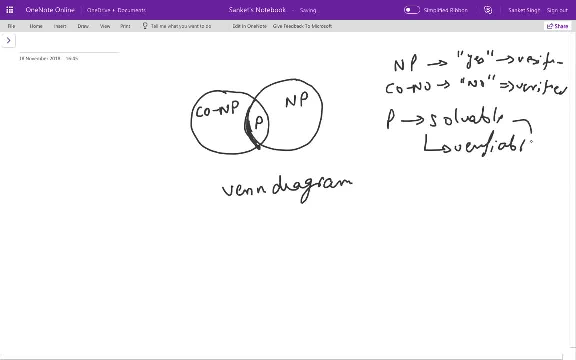 and verifiable both in polynomial time. so we can say that p lies as the intersection of the np and the co-np class. so now let us look at another class of problem that is called as np hard problems. but before describing the np hard problems, i want to mention a note here that the p class problems are also known as. 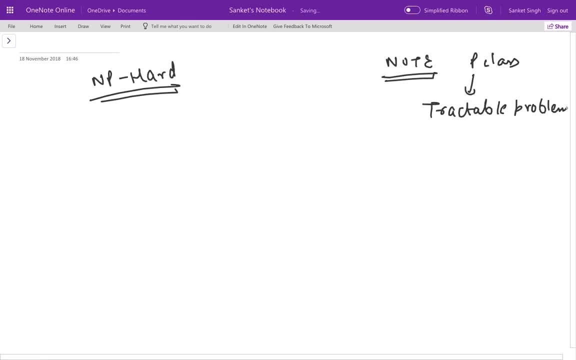 trapped table problems and the np class problems are known as also known as intractable or hard problems. so the p class problem is also called as the tractable problem and the np class problem are also known as intractable problems. so now let us look at a very new 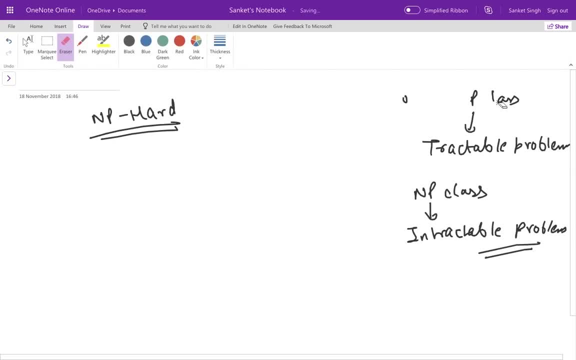 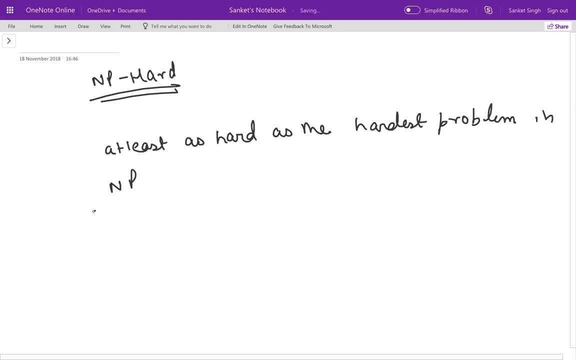 class of problems, that is np hard. so what an np hard problem is? an np hard problem is described as at least as hard as the hardest problem in NP. So what I'm trying to say? that a particular problem is called as NP hard if it is as hard as 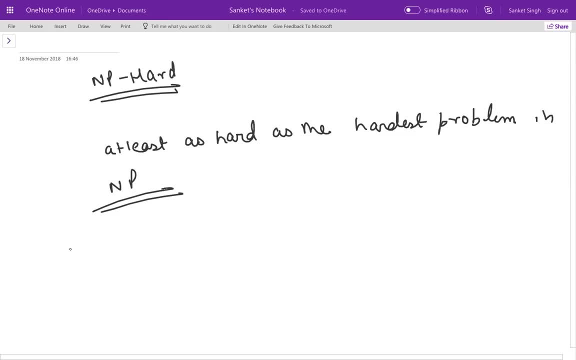 the hardest problem in NP. Suppose there is a problem x that lies in the NP class and this is the hardest problem in NP class. So what I'm trying to say by saying that a particular problem is hard is that it takes the maximum time in the verification of this particular NP problem. 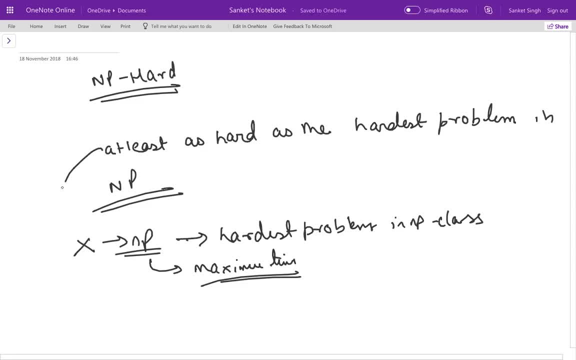 So if any problem is at least as hard as this particular problem, x, that lies in NP, then those problems lies in the NP hard class. So NP hard stands for non-deterministic polynomial time hard problems. So here you can see what I'm talking about is a non-deterministic polynomial time hard problems. So here you can see what I'm. 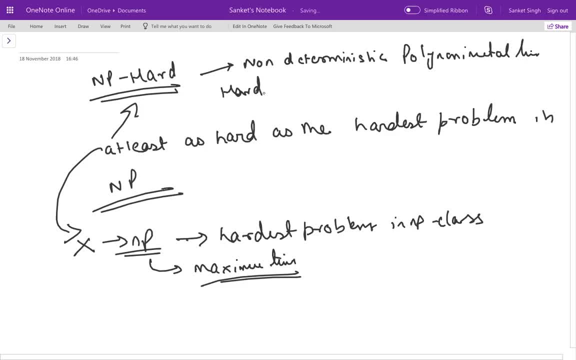 trying to say is that if a particular problem x that lies in the NP class is present and we have to define an another problem as NP hard, then this new problem should be as hard as the hardest problem in the NP class. It might be a fact that this new problem that was called as the NP hard problem is.